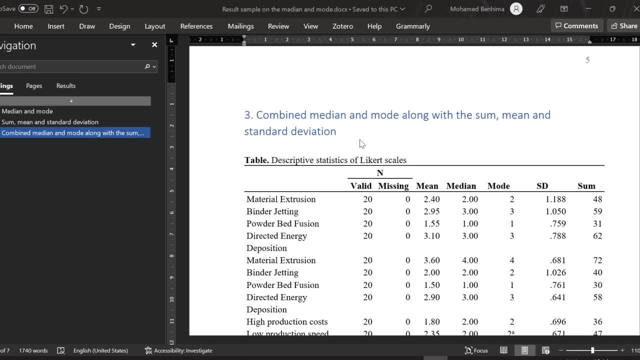 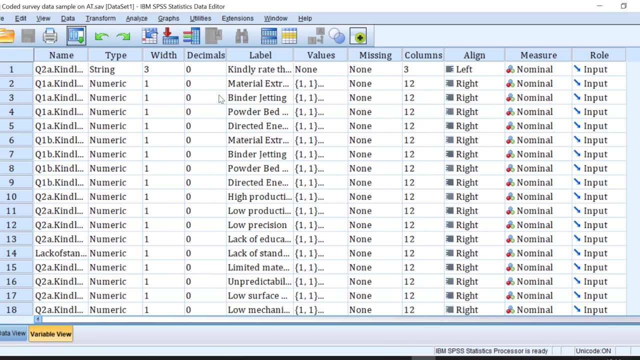 programs like Excel or whatever you want. So to do it using spaces, we need just to open the data sample here, this questionnaire, and we need to go to analyze. So this questionnaire is about different Lackert scale items that range from one to four or one to five, regardless of the scale We need to go to. 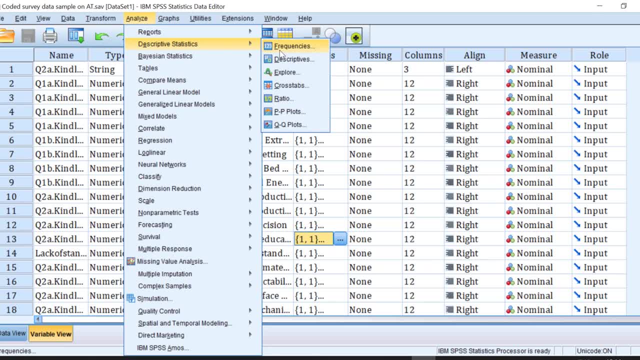 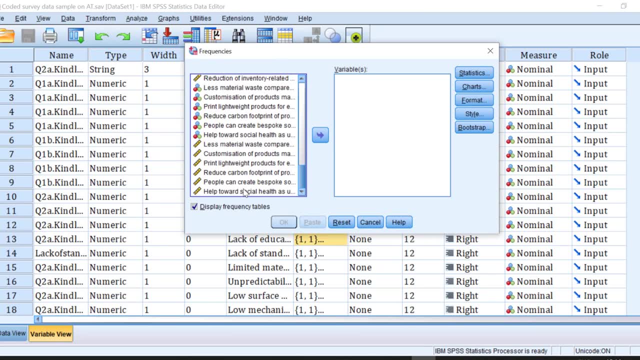 analyze, and then descriptive stats, and then frequencies. click frequencies and let's move all the items, the separate items together, to this box. As you can see, here the coding or the measurement level doesn't matter, It's nominal, It can be even ordinal or scale. 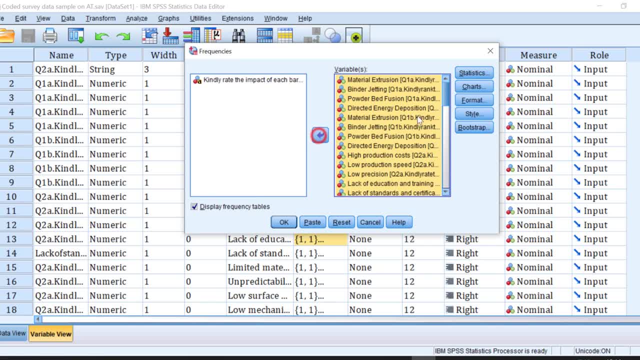 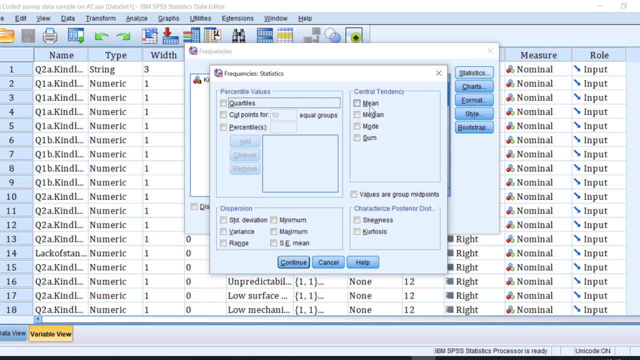 It depends on the objectives of your analysis. Let's move it here and let's end check display frequency tables. Let's go to stats and choose what we want to have like measures of central tendency and measures of dispersion as far as the descriptive stats are concerned. So for the 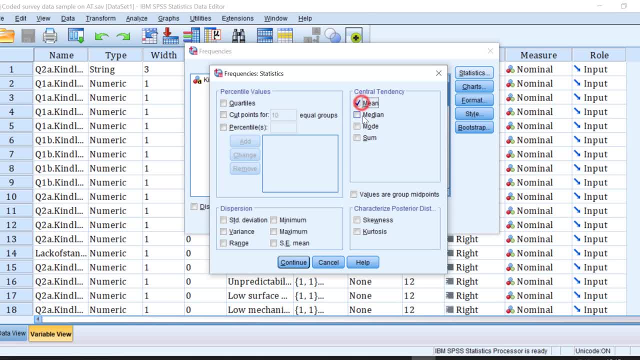 central tendency measure, I would like to have the mean, median and mode, and even the sum if I want so. And then for the dispersion measure, I want to have the standard deviation, That is how each respondent differs from the other in terms of the agreement or disagreement levels. 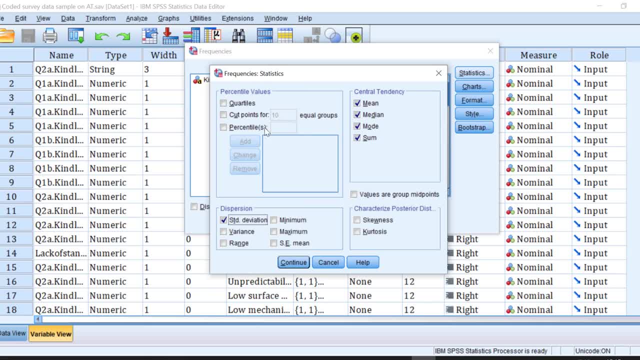 I can even choose the percentile or quartile levels. That's another thing. So I can literally choose whatever I want to have in the analysis from this box. I click continue and then click OK And let's wait for the output. So here is this table. 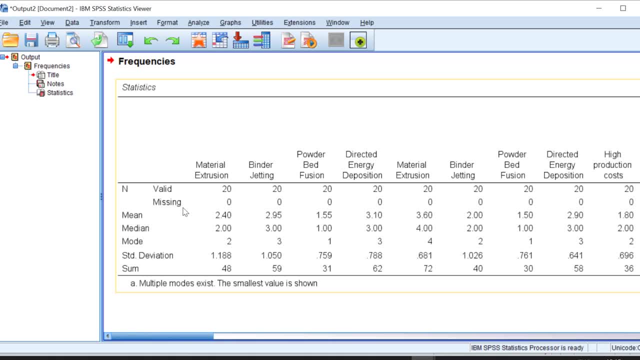 This table contains the sample size, the end, the valid along with the missing values, the mean score, the median score, the mode and the standard deviation along with the sum. So to take this table and copy and paste it to Word, that would look something that is. 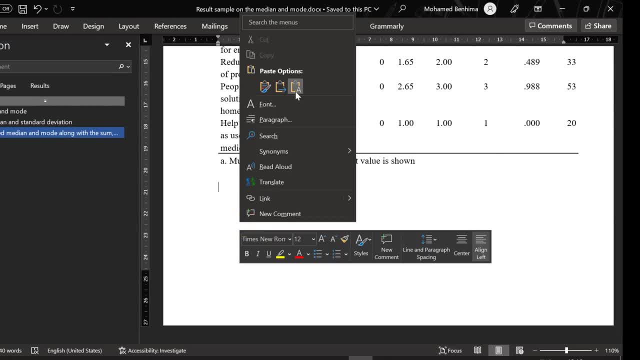 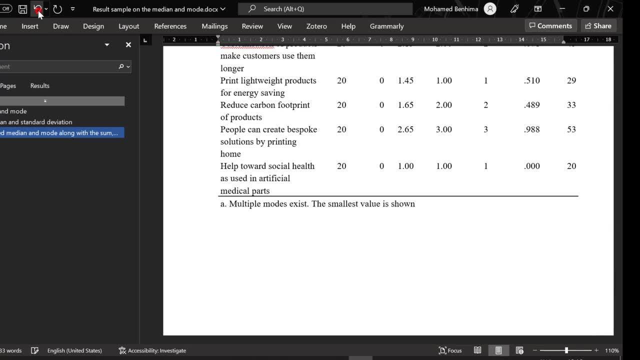 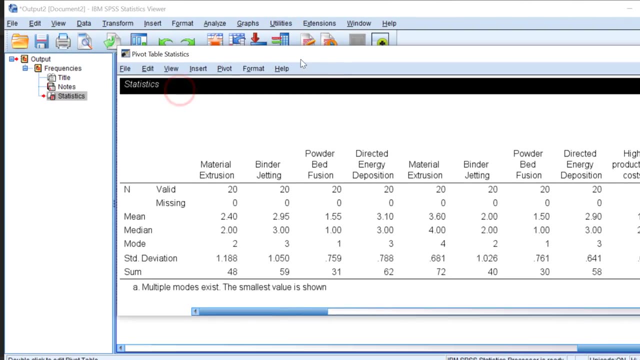 difficult, So it will be messy, as you can see. So what can we do to make it good or to make it look good? So to make it, let's say, look good, we need to go back to a space and I need to double click the table. This is left click. I need just to have this option and 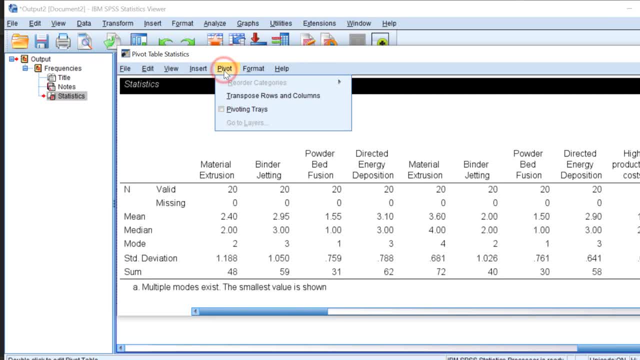 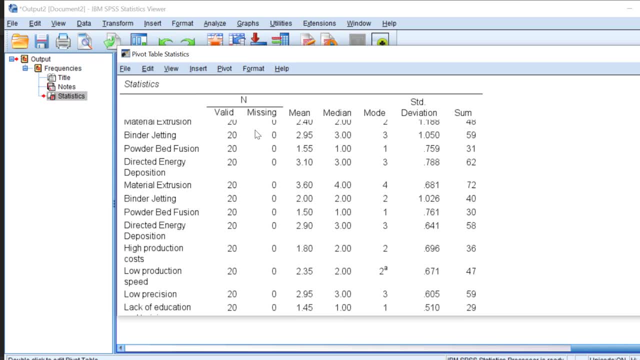 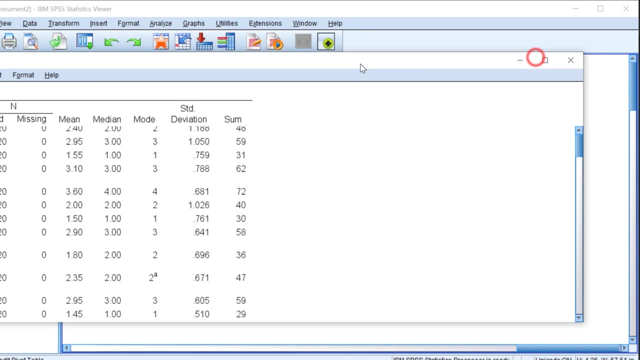 I have the private option. So I click the private option and I click transpose rows and columns. Click there and here you are. So we have the rows and columns transposed. And what we can do next? just let's click somewhere or just remove this box and go back to the output and let's click on it. 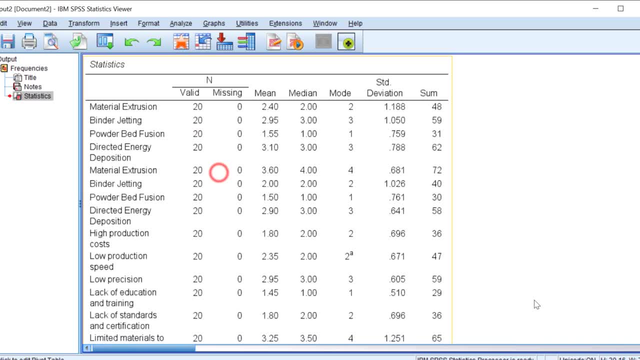 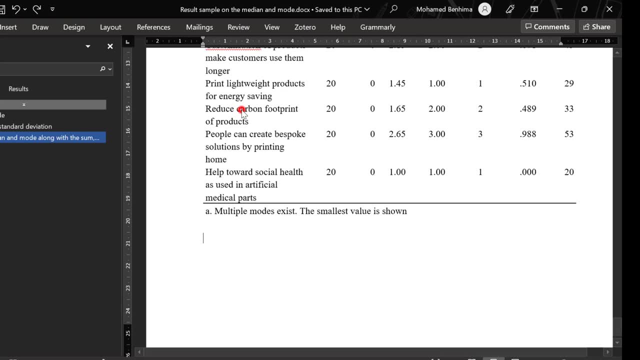 and right click And I need to double click the table. This is left click and I need to double click the page and I just go to copy and then go back to Microsoft Office Word and right click and then paste, So I can just keep source formatting. I need to change, for example, the font and the sum. 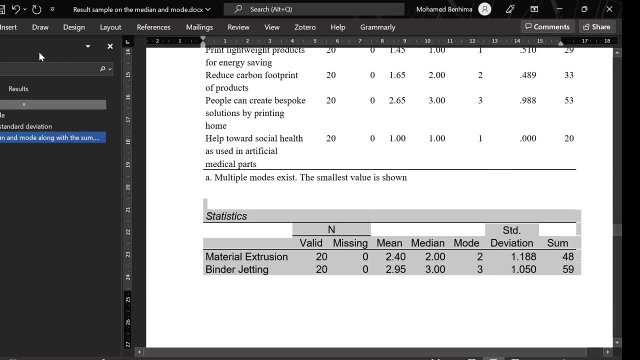 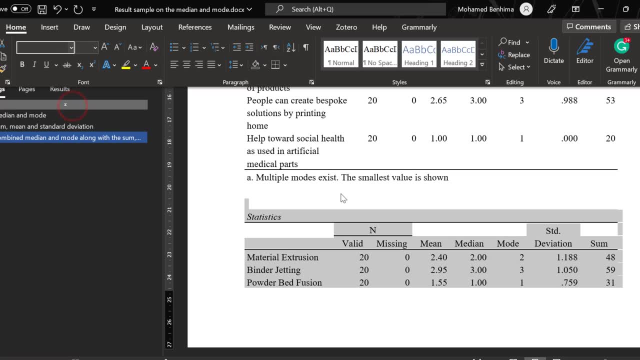 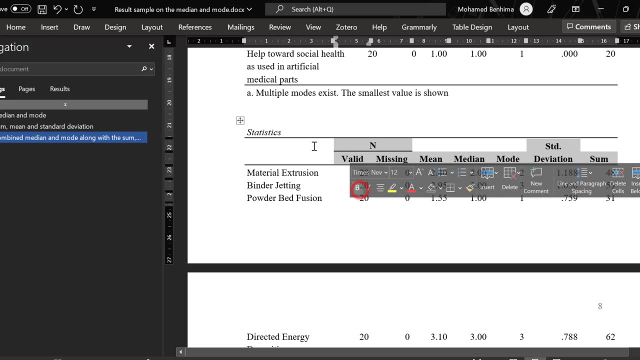 of the size just on Microsoft Office Word. That's really straightforward. I'll make it Times New Roman 12 according to the EPA style, and I can just, let's say, make that these things in bold. So I need just to keep formatting it the way I would like to to have it in the final version. so this is how. 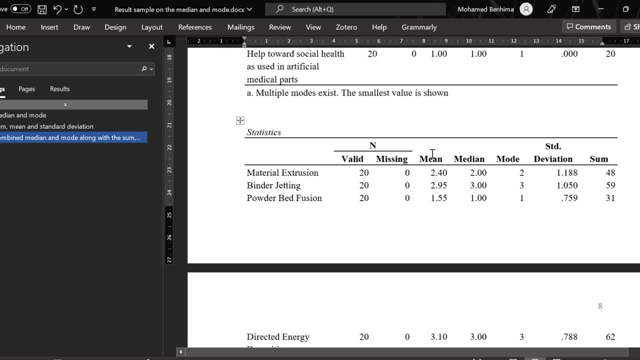 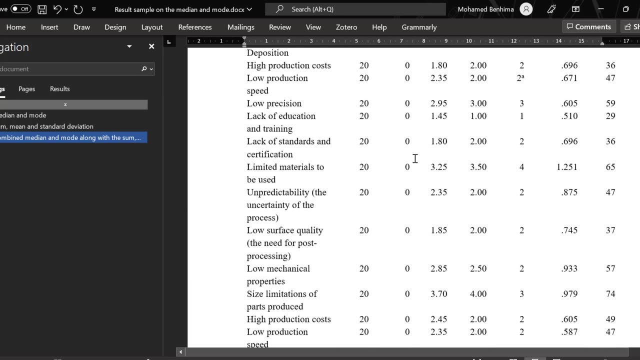 you can combine the different placards or the different descriptives, like the measures of central, tendency, of the mean, median and mode, and measures of dispersion like the standard deviation, the variance or even the standard error, in one table, and how you can write the results in. 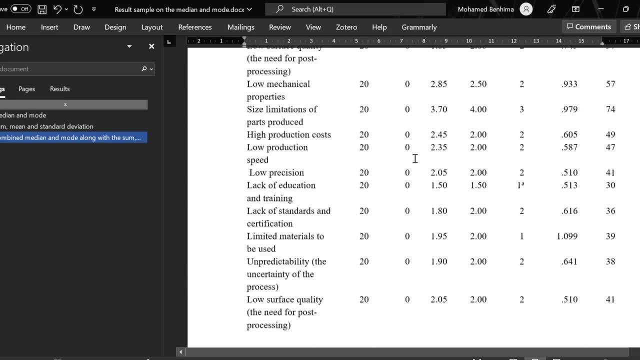 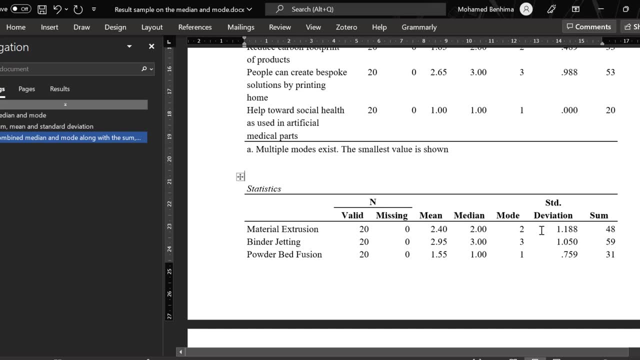 Microsoft Office Word. you can take whatever value. so for the mode, as I said, the most frequent, value two. this means that if the placard scale is coded from one strongly disagree to four strongly agree, this means that most respondents disagree with this first item. so the second one is: has received. 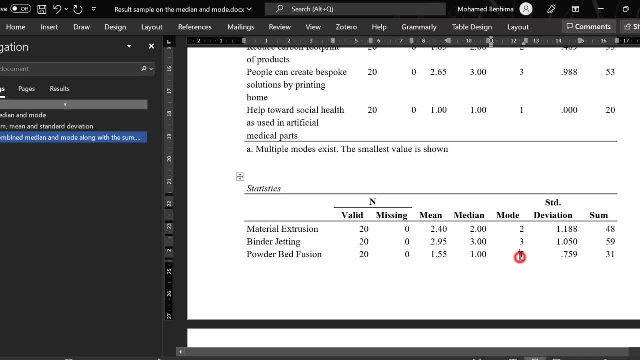 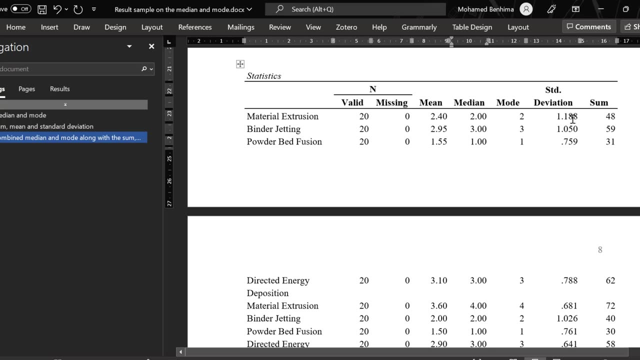 for example, neutrality, the first one disagreement. so this is how you can interpret the mode. that is the most frequent value. the median is the midpoint. the mean is the average. as I said, the higher the mean score, the more respondents agree. the lower the mean score, the less the respondents degree. the standard deviation refers how each respondent differs from the other. 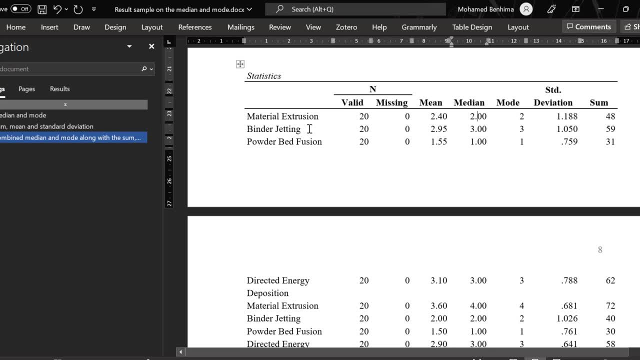 like if there is any homogeneity in terms of the agreement levels among the respondents, or there is this heterogeneity or divergence with regard to the attitudes expressed by respondents to the different placard scale items. the sum is sometimes used for some developed or adapted lacquered scales.